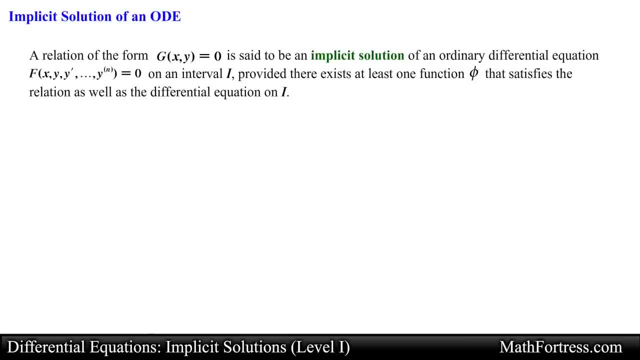 In general, a relation of the form g of x and y equals 0 is said to be an implicit solution of an ordinary differential equation on an interval i, provided there exists at least one function that satisfies the relation as well as the differential equation on i If 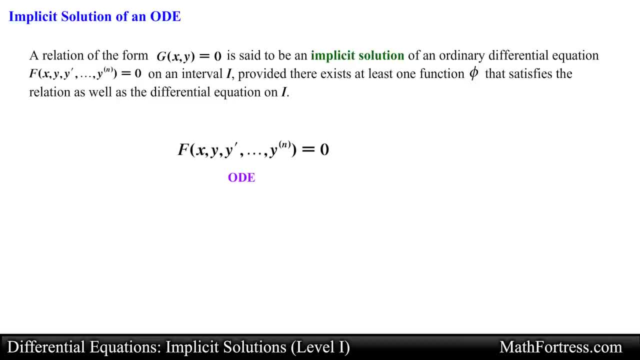 you happen to solve a differential equation and found a solution of the form g of x and y equals 0, then there exists at least one function that satisfies both the relation that is, g of x, of phi, of x equals 0, and a differential equation on. 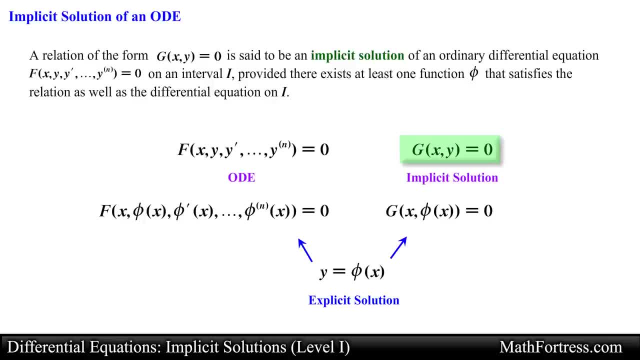 an interval i. At times, if the implicit solution is fairly simple, we may be able to solve for y in terms of x and obtain one or more explicit solutions. For the most part, there is usually no need or, as a matter of fact, the solution is pretty simple. 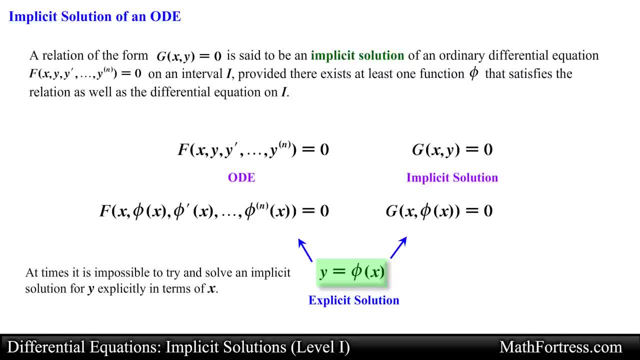 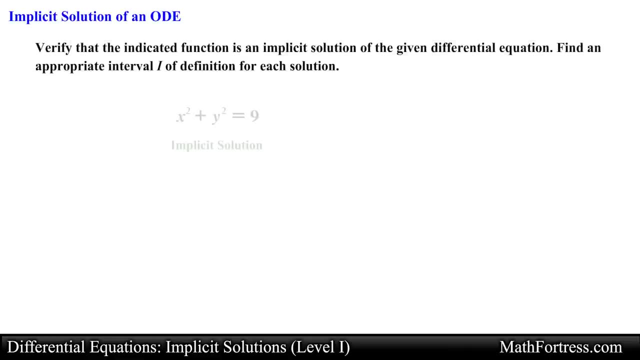 is just plain impossible to try and solve an implicit solution for y explicitly in terms of x. the best we can do is to numerically generate the graph of the solution and determine an appropriate integral of definition. For example, let's verify the following implicit solution: x squared plus y squared equals 9 and the differential equation to verify is: 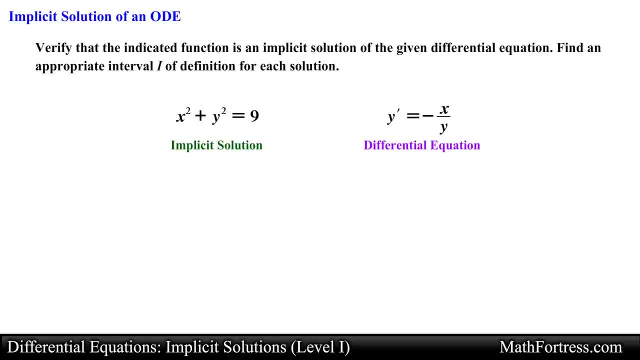 y prime equals negative x over y. Just the way we verify the explicit solutions of ODEs: we first need to find the derivative of the solution. Notice that we are going to have to find the derivative of this function by implicit differentiation. a technique first. 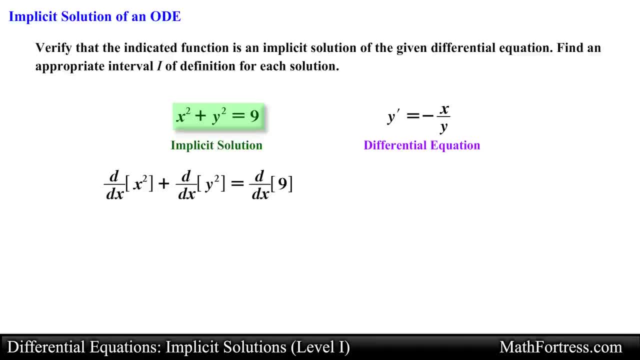 introduced way back in your differential calculus course. if you need a refresher, you can always look back at the calculus 1 videos. Alright, taking the derivative of this function implicitly with respect to x, we obtain the following expression: Now, if we were to solve for y prime, we would: 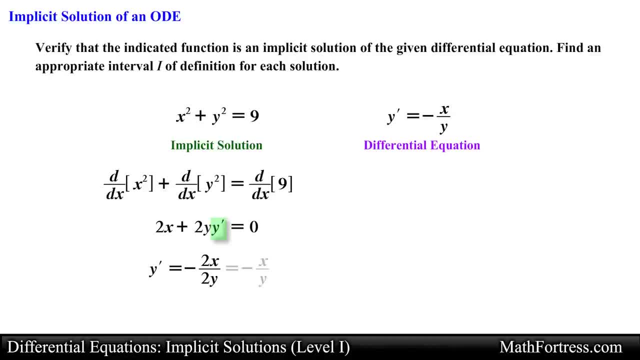 obtain the following Simplifying the expression, we see that y prime is equal to negative x over y. if we substitute y prime into the differential equation, we see that both the left and right hand sides match. hence this implicit function is a solution to the differential. 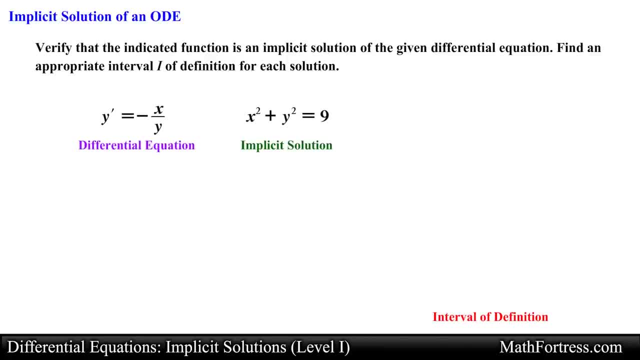 equation. Next, we need to find an integral I of definition To find this interval. let's go ahead and plot this implicit solution. Recall that this equation describes a circle with center located at and with radius equal to 3.. At first glance, you might be tempted to define the entire circle as your interval of definition. unfortunately, 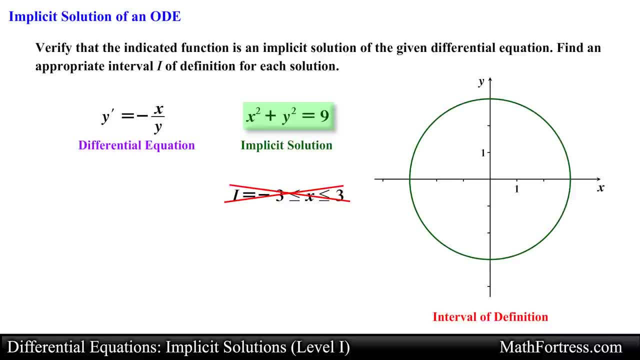 this would be incorrect. Recall that a solution to a differential equation has to be differentiable at the given interval i of definition. Notice that this function would not be differentiable at x equals negative 3 and x equals positive 3, because the tangent line at these points. 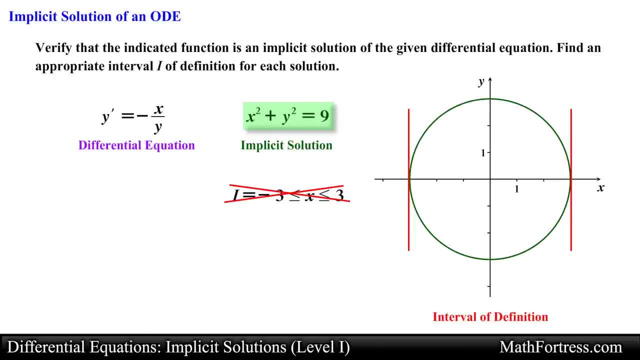 will be vertical and therefore undefined, meaning the implicit function is not differentiable at these points. As a result, we will need to label these points with open circles. Notice that this solution is now broken up into two semicircles. it turns out that we can actually: 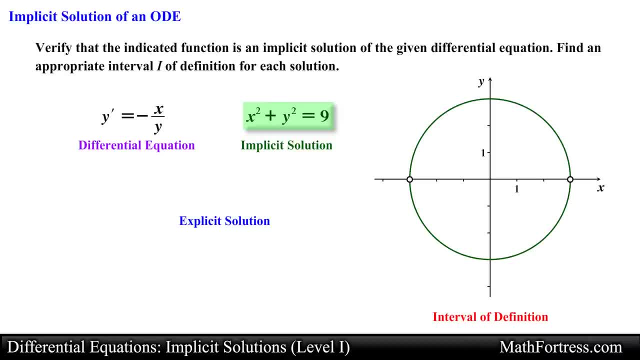 find an explicit solution to this differential equation. Let's take a look at the implicit solution. Notice that we are able to solve for y in terms of x. all we need to do is to isolate the variable y. doing that, we obtain the following expression: y equals positive, negative, the square root of 9 minus. 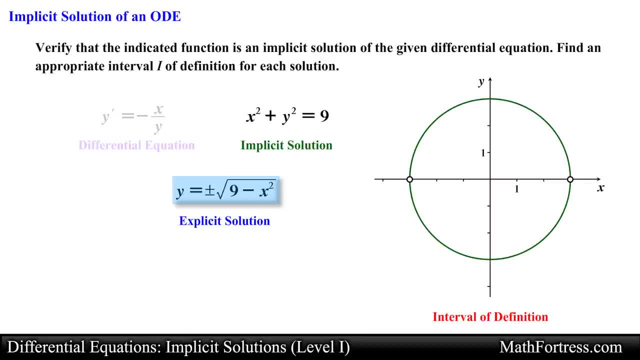 x squared. Notice that we were able to find two explicit solutions to the differential equation. the first is the positive square root of 9 minus x, squared, and the second is the negative square root of 9 minus x squared. Notice that these two functions satisfy the 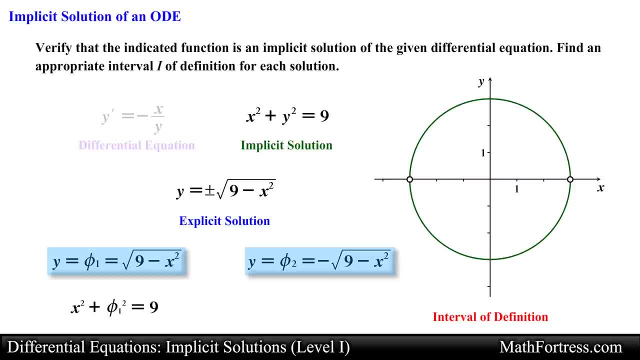 relation. that is, x squared plus the first explicit solution squared equals 9, and x squared plus the second explicit solution squared equals 9.. As well as the differential equation. Moreover, each explicit solution represents a segment of the implicit solution. The first explicit solution forms the top semicircle and the negative explicit solution forms the bottom. 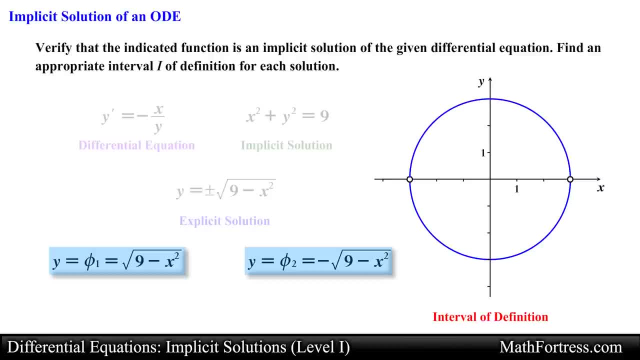 semicircle. In addition, notice that the domain of the explicit solution is defined from negative 3 inclusive to positive 3 inclusive, but, as we just saw, in order to satisfy the differential equation, these solutions can't be defined at x equals 3 and x equals negative 3.. As 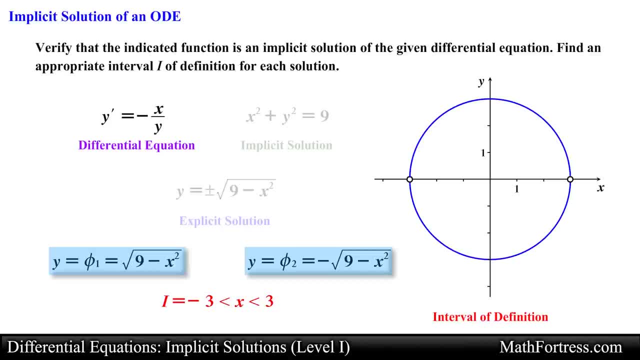 a result, we have two options for our interval of definition. we can use the first explicit solution and define our interval of definition from negative- 3 exclusive- to positive- 3 exclusive, or we can use the second explicit solution and define our interval of definition from: 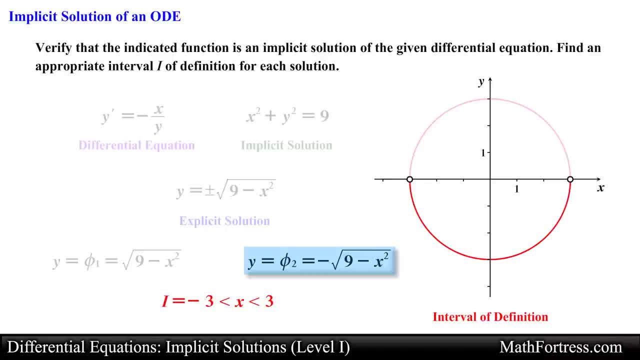 negative- 3 exclusive- to positive- 3- exclusive. either of these intervals can be used as our interval of definition. In a much later video, we will be required to choose one interval over the other. for now, either of the explicit solutions, along with their intervals, are acceptable. 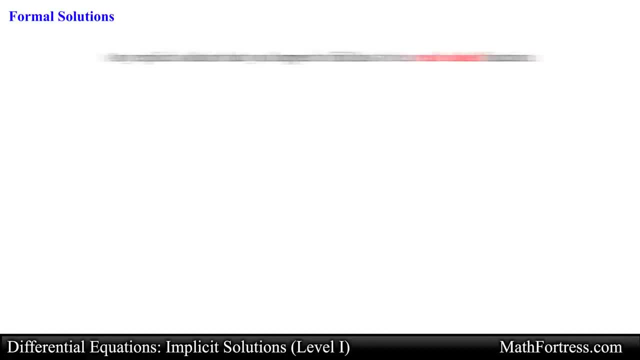 answers. The final thing I want you to be aware of when dealing with implicit solutions is to make sure that any explicit solution that you happen to find has to be a real valued function. For example, say that we are asked to verify the following implicit solution: x squared plus y squared equals negative. 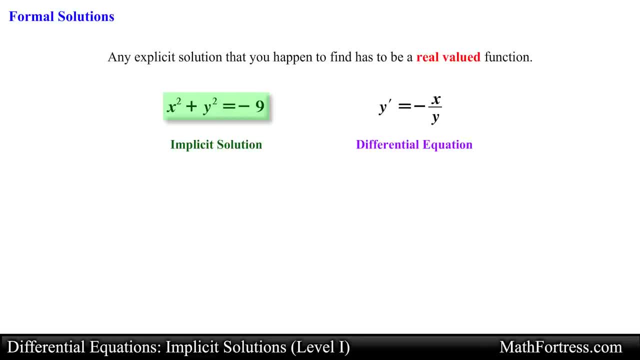 9, notice that the only difference between this implicit function and the one from the previous example is that this one is equal to negative 9.. If we were to solve for an explicit solution, we would obtain the following expression: y equals positive, negative, the. 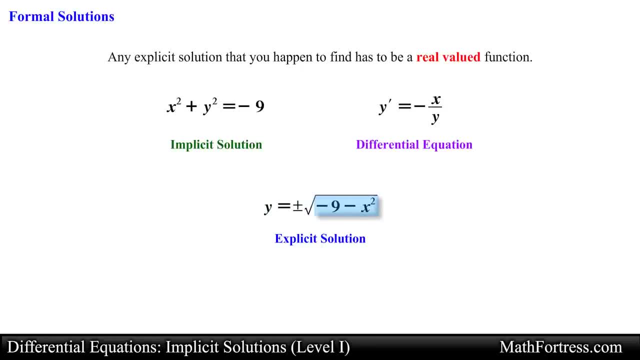 square root of negative 9 minus x squared. Notice that any value of x will force us to take the square root of a negative number and therefore we are unable to draw a graph of this function, since it is not a real valued function. Although the explicit solutions are not real valued functions, they nevertheless. 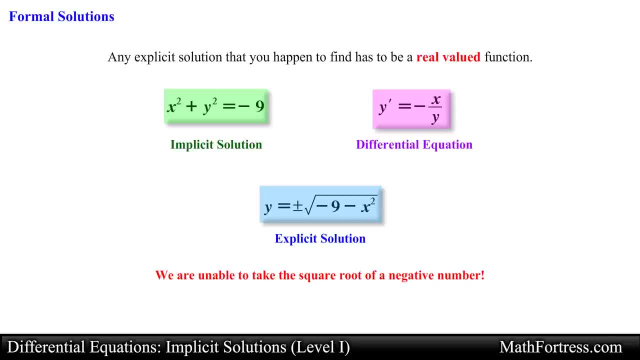 satisfy the relation and they also satisfy the differential equation. so we have to be careful when finding explicit solutions of implicit relations. The implicit solution might satisfy the differential equation, but an interval of definition cannot be determined because the explicit solution is not a real valued function. When this occurs, we say that the implicit relation is a formal solution. 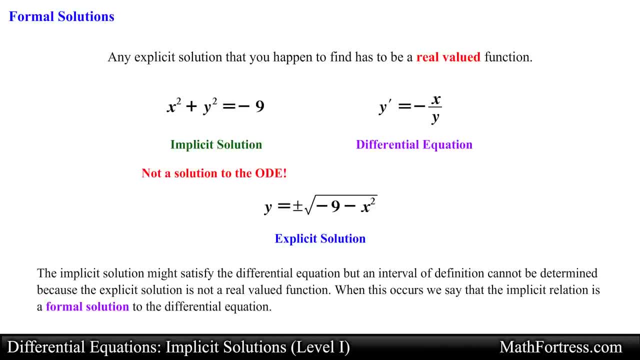 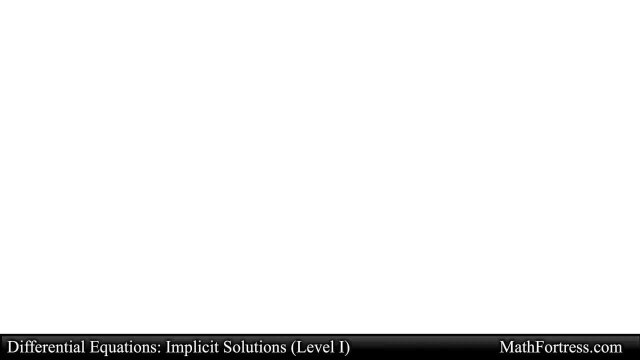 to the differential equation. Keep in mind that the implicit relation is not a solution to the ODE, since no interval of definition can be defined in any interval, but the relation just happens to formally satisfy the differential equation. Alright, to sum up, A solution of the form y equals phi of x is called an explicit solution of an ordinary.